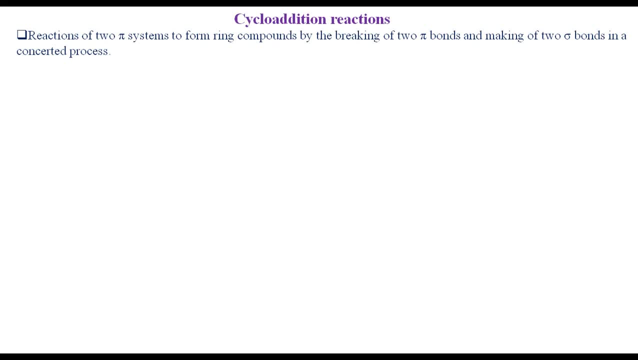 These are the reactions of two pi systems to form ring compounds by breaking up two pi bonds and making of two sigma bonds in a concerted process. The reverse of cycloaddition reactions are known as retro cycloaddition reactions. Typical examples are the conversion of two 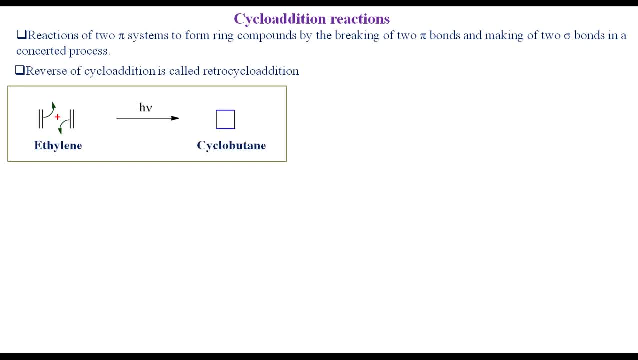 molecules of ethylene into cyclobutane and reaction of 1,3-butadiene with ethylene to produce cyclohexene During cycloaddition reactions of two ethylene molecules. the reaction of 1,3-butadiene to ethylene to produce cyclohexene During cycloaddition reactions of two ethylene molecules. 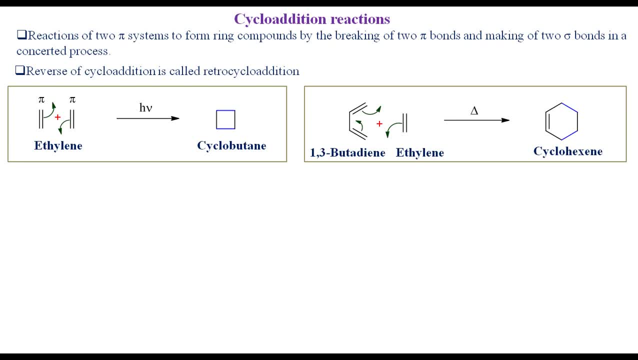 two pi bonds are consumed In replacement. two sigma bonds in the product. cyclobutane are formed. Similarly during the cycloaddition reaction of 1,3-butadiene and ethylene. two pi bonds of the reactants, one from each, are consumed to form two sigma bonds in the product. 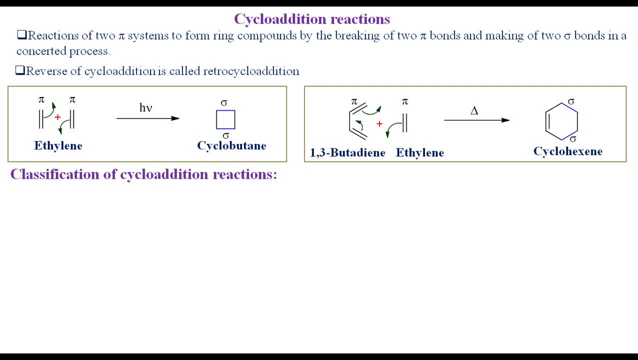 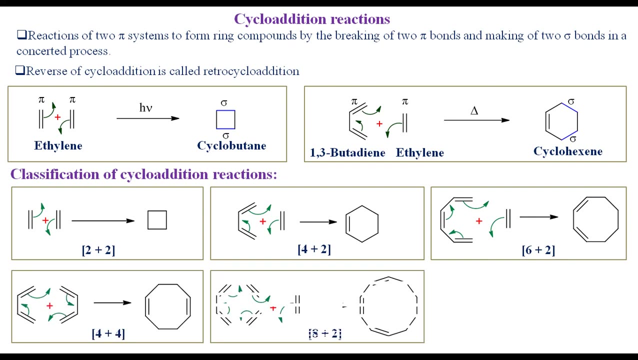 Based on the number of pi electrons of the reacting species involved during the reaction. cycloaddition reactions have been classified as 2+ 2, 4+ 2, 6+ 2, 4+ 4, 8+ 2, 6+ 4,, etc. 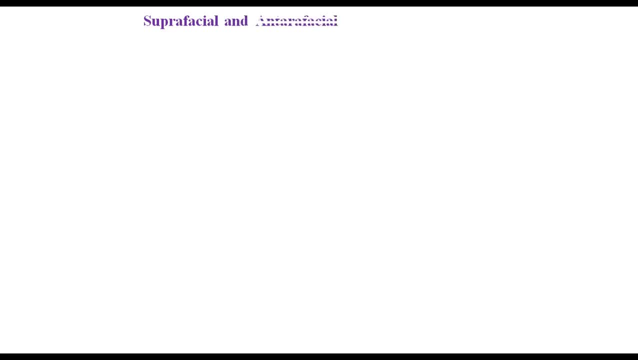 Now we will learn two terminologies which will be used for the derivation of Woodward-Hoffmann selection rules for cycloaddition reactions. Now we will learn two terminologies which will be used for the derivation of Woodward-Hoffmann selection rules for cycloaddition reactions. 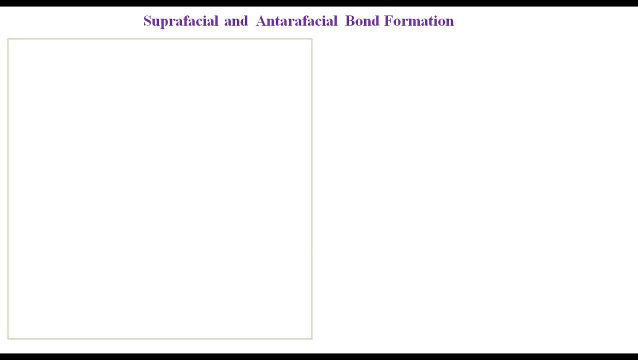 For the cycloaddition reaction to occur, HOMO of one reactant interacts with the LUMO of other. Positive terminal lobe of one can interact with the positive terminal lobe of other, and negative terminal lobe of one can interact with the negative terminal lobe of other. 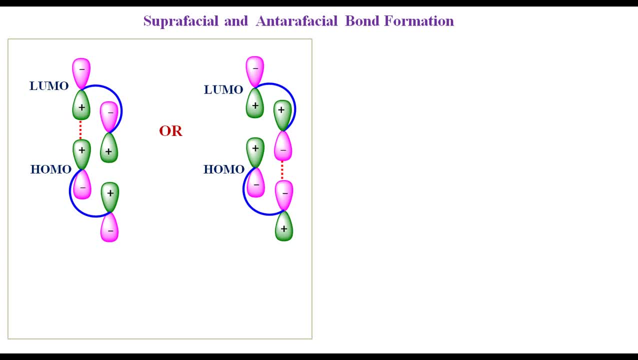 If the structure of HOMO and LUMO of the two reactants is such that bonding interactions occur between the lobes on the same face of one reactant and the lobes on the same face of other, the interaction is called supraphacial interaction. 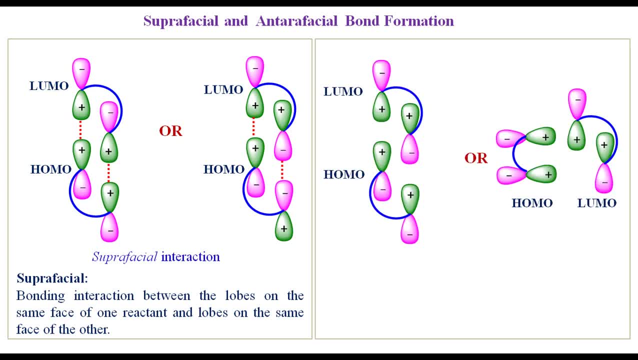 If the structure of HOMO and LUMO of the two reactants is such that bonding interactions occurs between the lobes on the same face of one reactant and lobes on the opposite faces of the other, the interaction is called entorhapacial interaction. 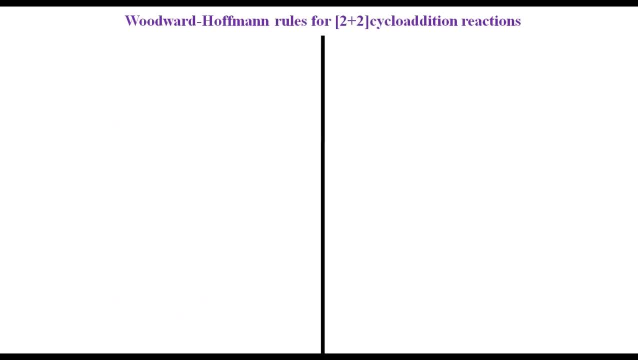 Now let us derive the Woodward-Hoffmann selection rule for 2 plus 2 cycloaddition reaction. In the previous lecture, ie Electrocyclic part 1,, we have already learnt how to make Haeckel molecular orbital diagrams for ethylene and different conjugated pi systems. 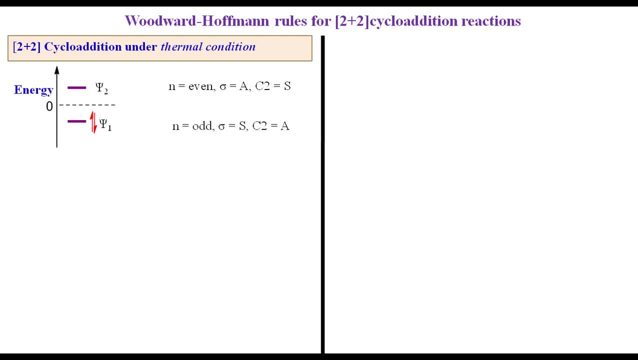 In ethylene there are two pi molecular orbitals, psi1 and psi2.. Under thermal condition, psi1 is fully occupied by two pi electrons and psi2 is fully vacant. So psi1 acts as HOMO, while psi2 as LUMO. 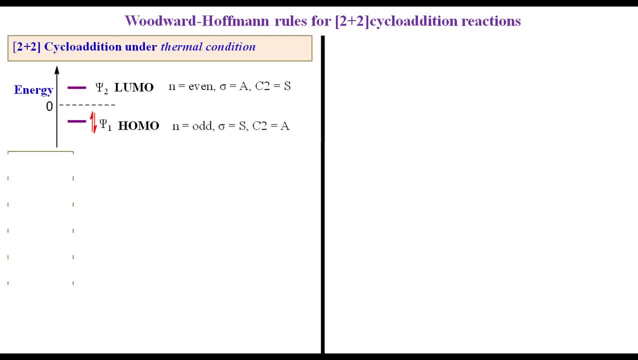 During cycloaddition, HOMO of one ethylene molecule combines with LUMO of other. Since HOMO and LUMO have the same number of electrons, the HOMO of one ethylene molecule acts as HOMO and LUMO acts as LUMO. 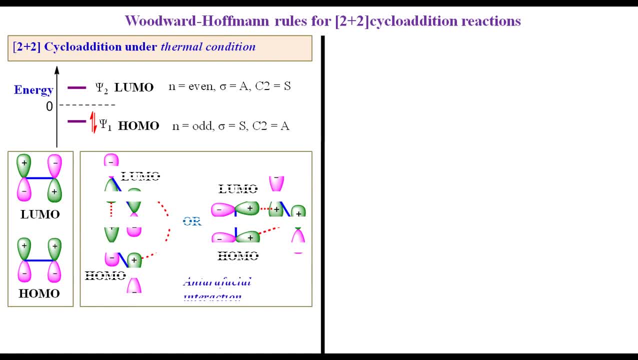 During cycloaddition, HOMO of one ethylene molecule combines with LUMO of other. Since HOMO and LUMO have two different symmetries, so the allowed bonding interaction will be antarafacial, which is not possible in small ring systems like cyclobutane. 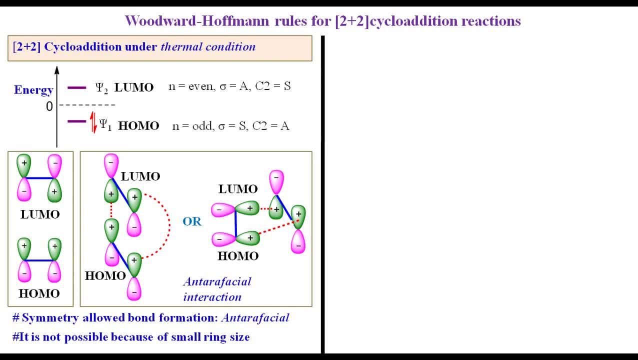 So 2 plus 2 cycloaddition is thermally not allowed Under photochemical condition. one of the two pi electrons from psi1 jumps to psi2, making psi2 as HOMO Under thermal condition. HOMO from psi2 is always allowed because psyche is not an inorganic. 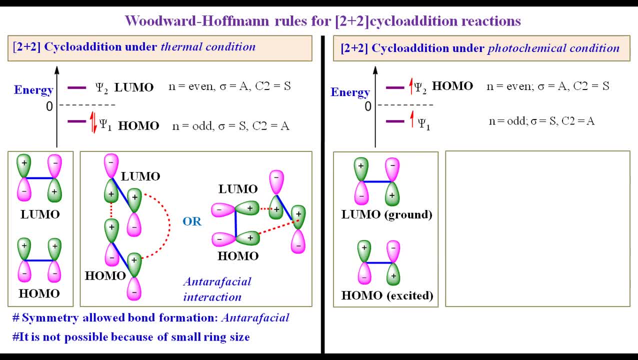 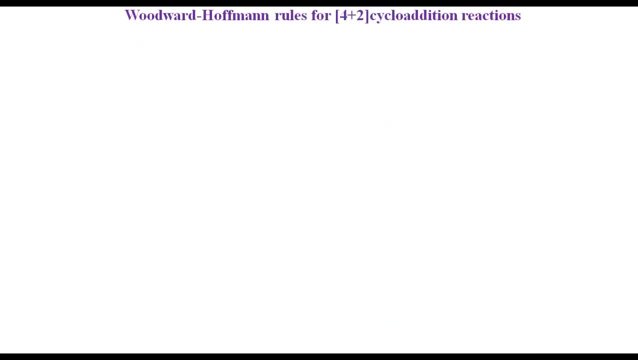 particle. In the case of HOMO, the HOMO in the form of HOMO is not the HOMO which is not inorganic particle. In the case of HOMO, HOMO is not the HOMO which is not inorganic particle. 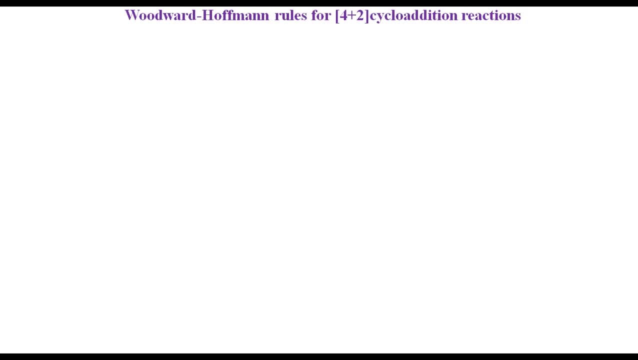 So HOMO is not an inorganic particle. This is just a processing of HOMO. These two pi electrons are not inorganic. HOMO is not a single nucleic acid. These are single nucleic acid In 4 plus 2 cycloaddition under thermal condition. Psi 2 and Psi 3 of 1,3-butadiene are HOMO. 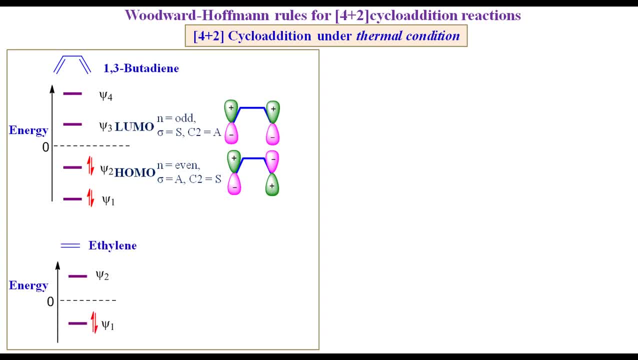 and LUMO respectively In ethylene. Psi 1 is HOMO and Psi 2 is LUMO. If we look at the structure of HOMO and LUMO of 1,3-butadiene and ethylene, we will find: 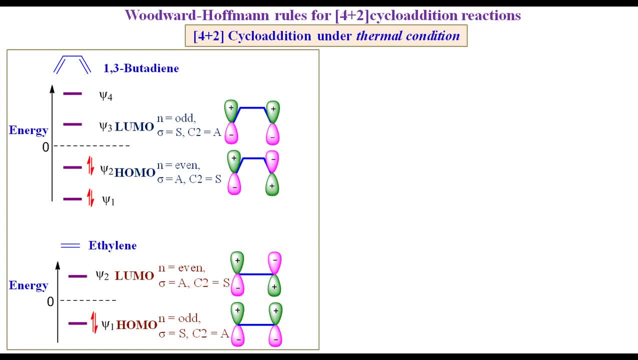 that HOMO of 1 and LUMO of other have the same symmetry. Thus HOMO of 1,3-butadiene can combine with the LUMO of ethylene, or HOMO of ethylene can combine with the LUMO of 1,3-butadiene in a supra-facial fashion. 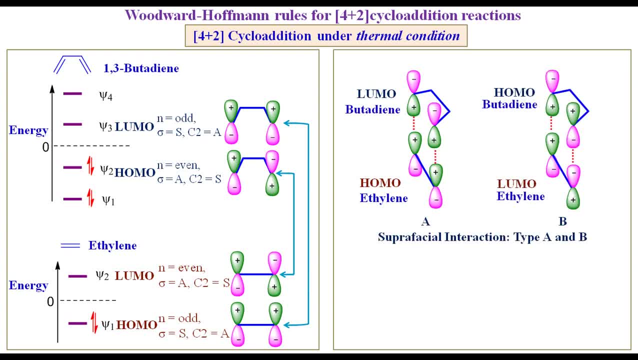 But in general interaction between HOMO of 1,3-butadiene and LUMO of ethylene is energetically more favorable because of the smaller energy gap between these two molecular orbitals. So 4 plus 2 cycloaddition is thermally allowed. 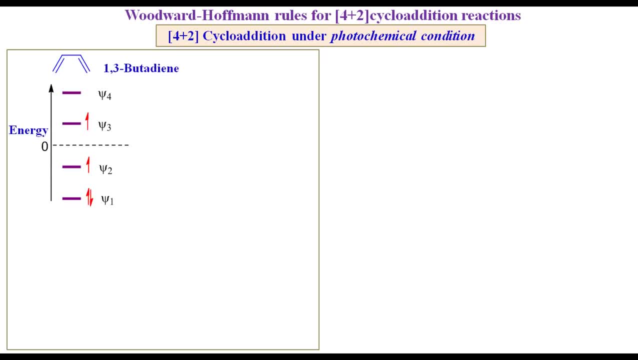 Under photochemical condition. one of the two electrons from Psi 2 of 1,3-butadiene jumps to Under photochemical condition. One of the two pi electrons from Psi 2 of 1,3-butadiene jumps to Psi 3,, making Psi 3. 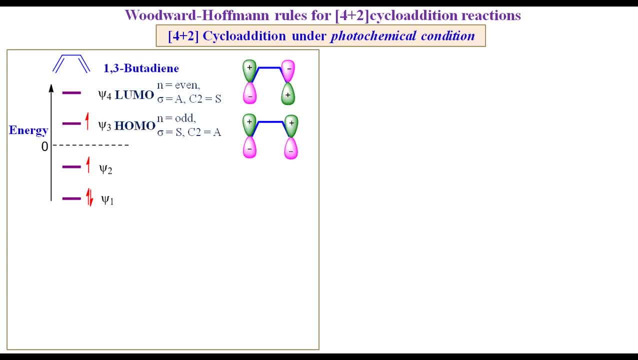 as HOMO and Psi 4 as LUMO In ethylene. Psi 1 is HOMO, while Psi 2 is LUMO. The HOMO of butadiene and LUMO of ethylene have different symmetry, so the allowed interaction. 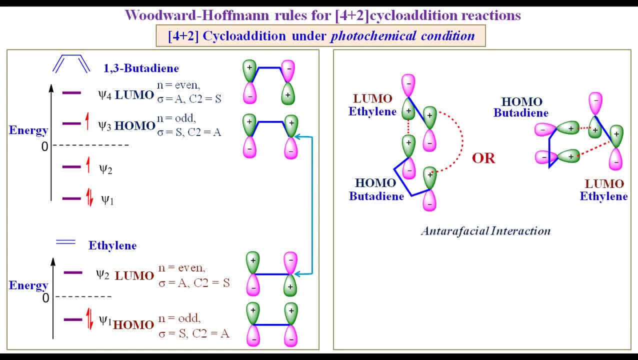 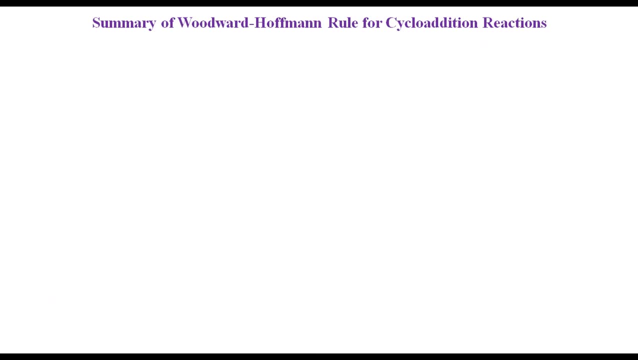 will be entera-facial. The molecule resulting from the entera-facial interaction will be: 2 is tend to be formed, So 4 plus 2. cycloaddition is photochemically not allowed. Based on the previous discussion, we can summarize Woodward-Hopman rule for cycloaddition reaction.